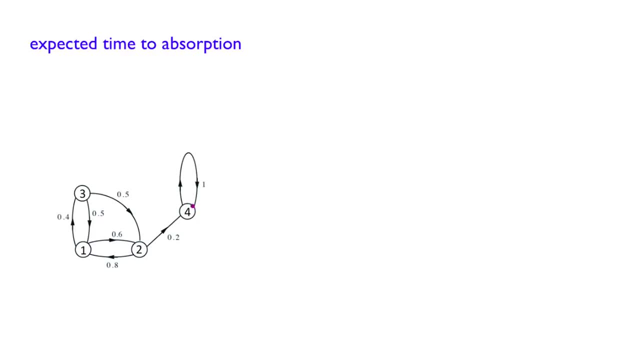 have to do until you reach 4?? Of course we don't know. It is a random variable. In fact, it's more than one random variable. It will depend probably on where you started, Starting from 2,, 1, or 3, or 4 would. 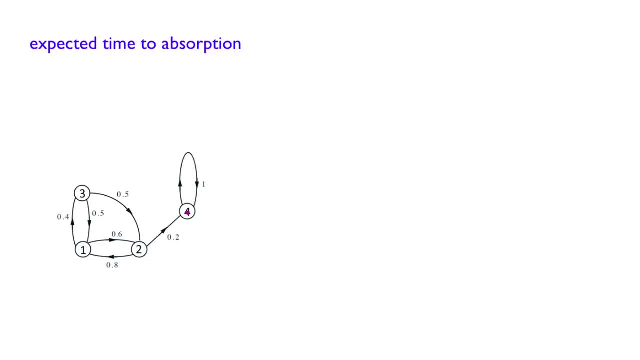 lead to different random variables. We are going to be interested in looking at their expectation, Or the expected value of these random variables. More precisely, let us define exactly what we want to do, which is to find the expected number of transitions that we're going to call mu of i, until reaching 4, which 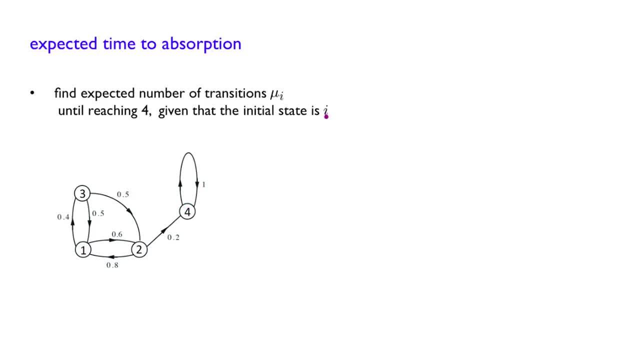 is our absorbing state, given that the initial state is i, one of these four states. First, as a warm-up, let's do some quick calculation. If you didn't have this part here and instead we were looking just at this portion here, 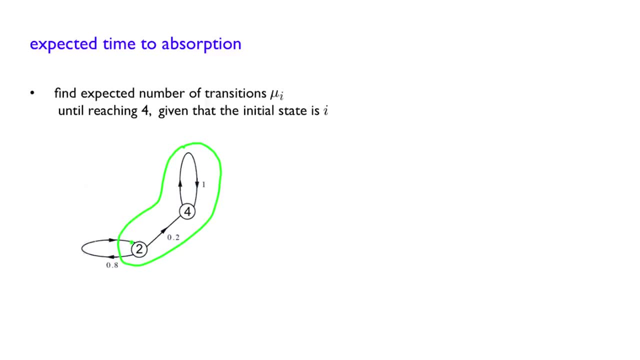 And make this one disappear like this And replace it by a loop of probability 0.8.. So now, if you start from state 2,, with probability 0.2, you will go to 4.. Or with probability 0.8, you will remain in 2.. 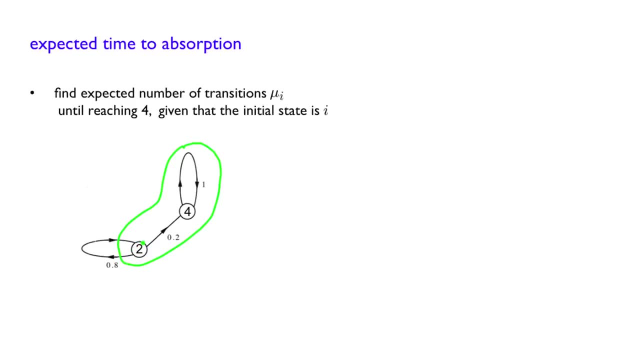 And now you ask yourself what is the number of trials you have to do until you reach 4?? Well, We know what it is. This is a geometric, random variable with the probability of success, which is a success being going to 4, of 0.2.. 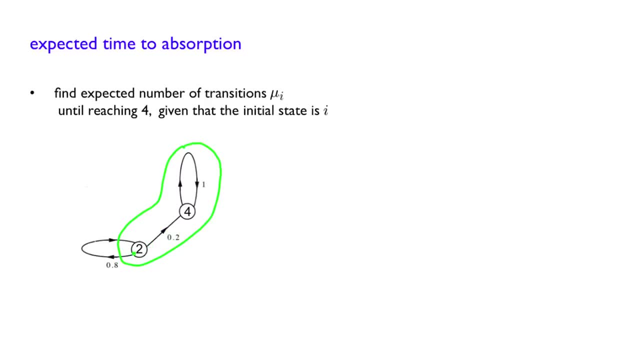 So the expected number of trial, starting from 2, that you will have to go through until you reach 4, will be 1 over this probability, So 1 over 0.2,, which is 5.. Now that we have done this quick calculation, 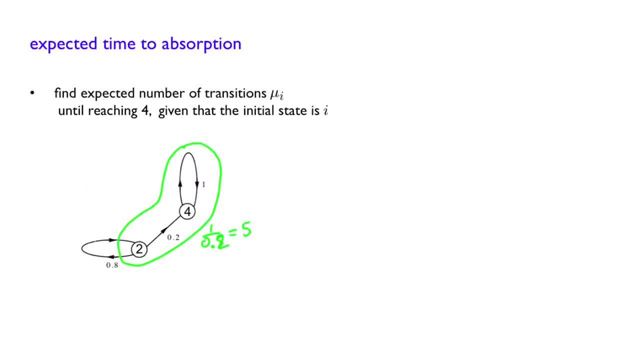 it should be clear that if we go back to the previous Markov chain that we had here, the expected time mu 2, will probably be bigger than 5.. Since from 2, not only you have the probability of going to 4,. 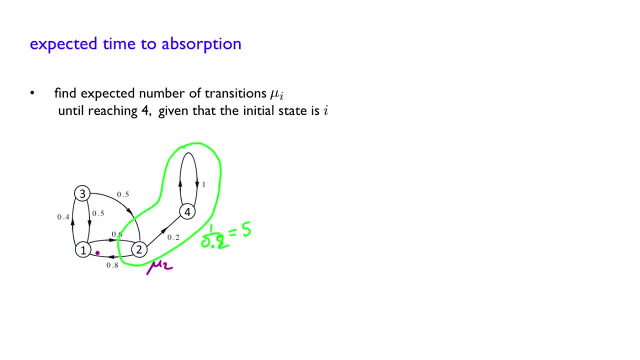 but you might have some chance of traveling there. So probably the number of time until you reach 4 will be bigger than 5.. Let us see Well, first of all, if you start at 4, the expected number of transitions until reaching 4,. 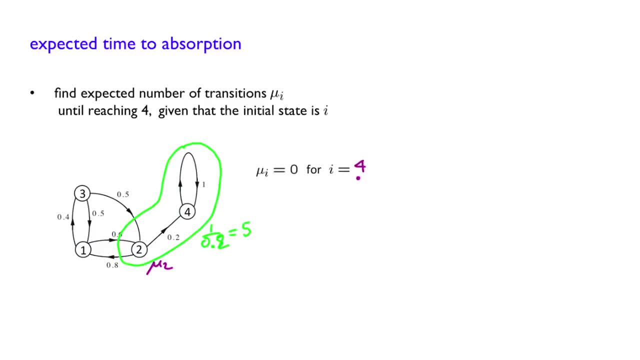 will obviously be 0. So here for i equals 4, you indeed get 0.. What about for the others? Well, again, this is what we would like to calculate. How are we going to do that? Well, the argument is going to be of the same nature. 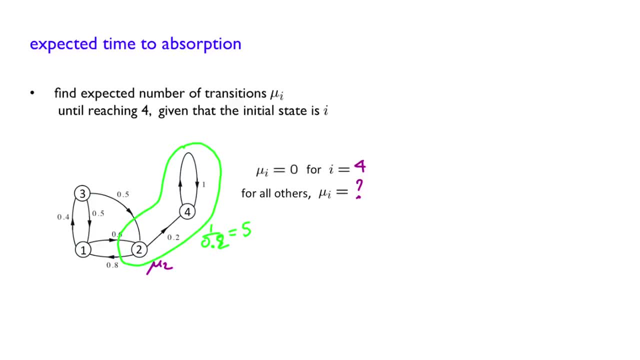 as the one that we used before. We are going to think in terms of tree and consider possible options starting from a given state. So let's do this calculation from 2.. So you are 2. And we're going to build that tree here. 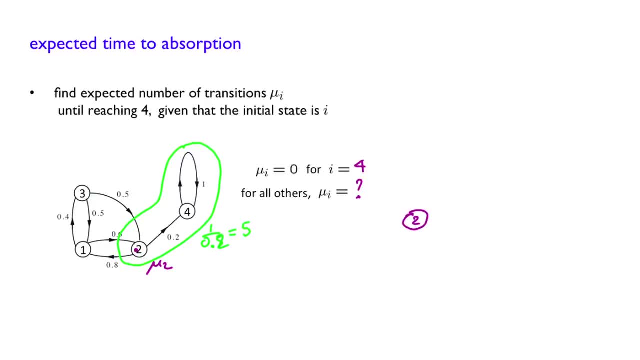 So you are in state 2.. What could happen next? Well, you can either transition to 4 with the probability 0.2, or with the probability 0.8,. you end up in 1.. And you have done one transition here, so plus one transition. 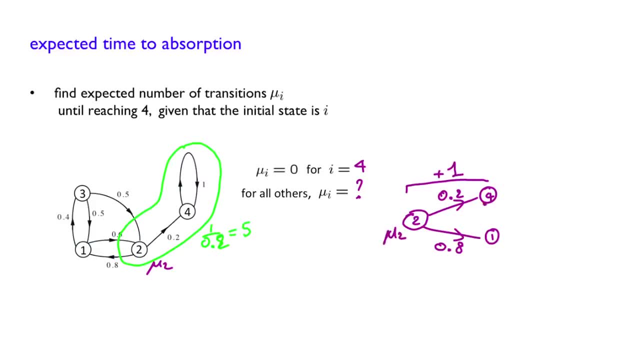 So you are interested in calculating mu 2.. After one transition you either end up in 4.. In that case you stop, You're done, Right. In other words, the resulting value here would be mu 4, which we know is 0.. 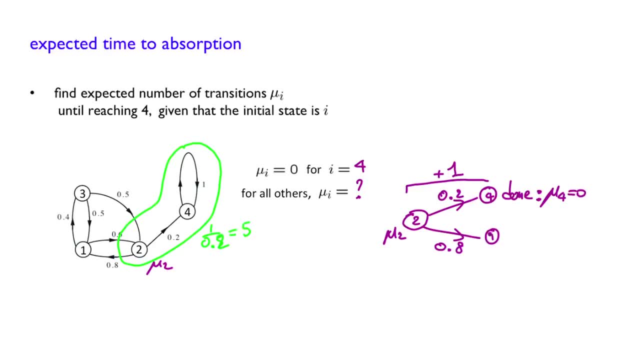 Or you are in 1.. And now, given that you are in 1,, you want to find the expected number of transition until reaching 4, which is exactly defined here. So here what you have is mu 1.. And now you can use the total expectation theorem. 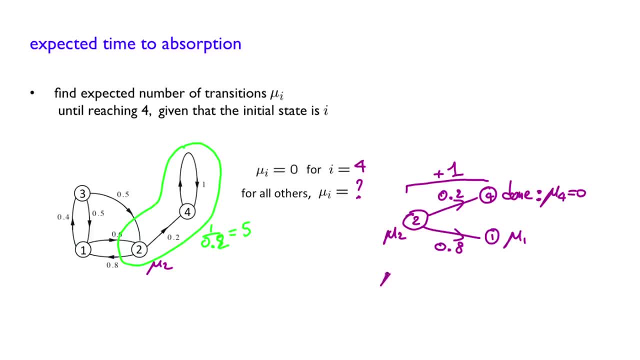 to put all of these things together, which what it means is that mu 2 will be 0.2.. Mu 2 will be 1.. You have one transition And then, after you do that transition with priority, 0.2,. 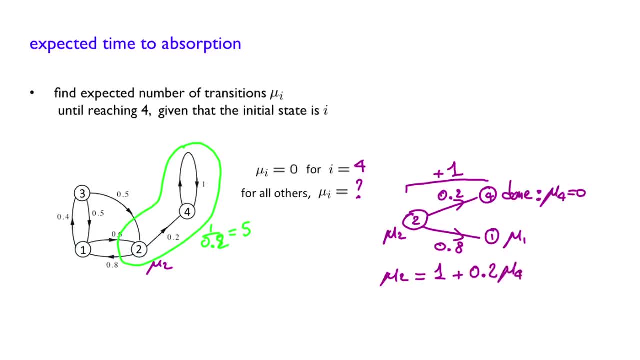 you know that you're going to be in 4. And the expected value then will be mu 4, plus 0.8, which is the priority, that you end up in state 1. And condition on that, the remaining expected iterations. 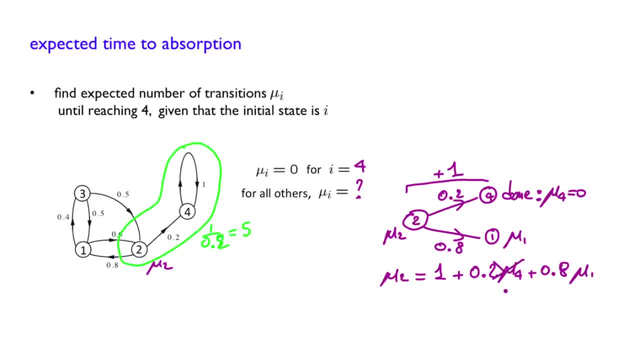 until reaching 4 will be mu 1.. Now this one here. This one is, of course, 0.. So what you end up is 1 plus 0.8 mu 1.. So you get a relation between mu 2 and mu 1.. 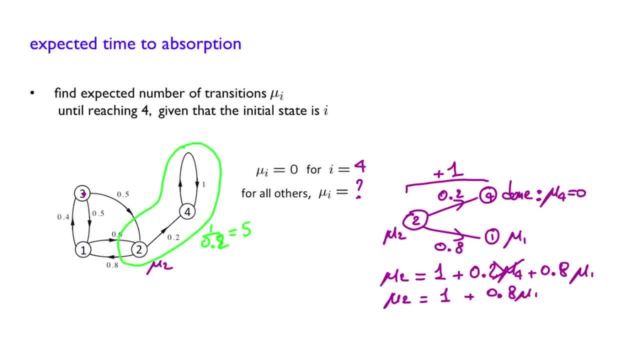 Now you can do the same thing if you start from 1 or start from 3.. So let's do it again From 1, so you're interested in 1.. After one transition, so plus 1, what happened? 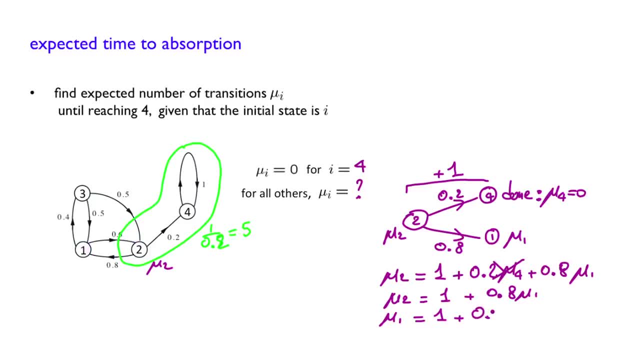 Well, with the priority 0.6.. You end up in 2.. And with the probability 0.4, you end up in 3.. And from 3, if you start in state 3, after one transition. what happened? 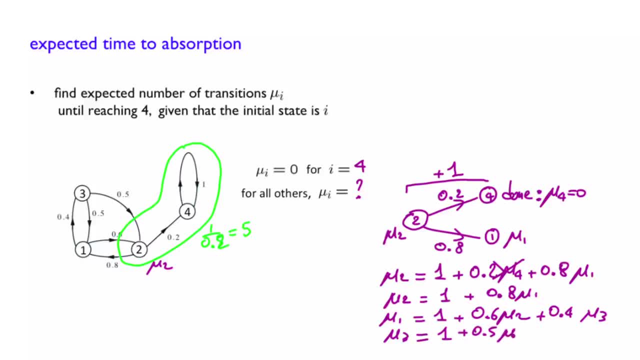 Well, with the priority 0.5, you would end up in state 1.. And then the expected number of transition from state 1 until reaching 4, it will be mu 1.. Or with the priority 0.5, you end up in 2.. 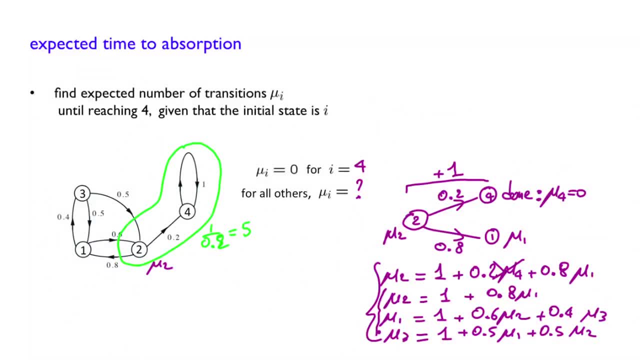 So again here, if you look at these three here, this is a system of three equations, three linear equations with three unknowns, And it has a unique solution. I will let you do the calculation. Let me give you the result. What you obtain is mu 1. 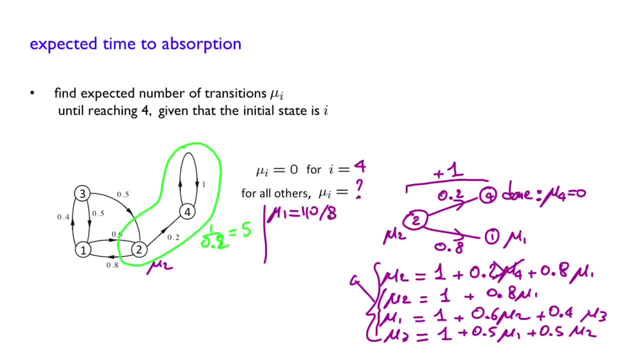 will be 110 over 8.. I'm writing it this way so that we can compare them. Mu 2 will be 96 over 8, which is 12. And mu 3 is 111 over 8.. So here again, a quick sanity check. 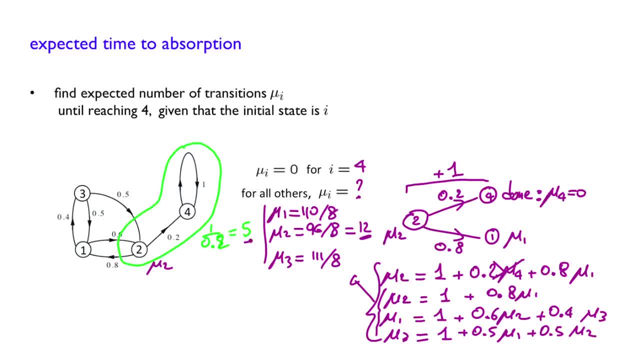 The number that we get here- 12, is indeed bigger than the 5 that we have obtained when we restricted ourselves to this set. So we do have mu 2 greater than 5.. Now, as the relative value between mu 1, mu 2, and mu 3,, 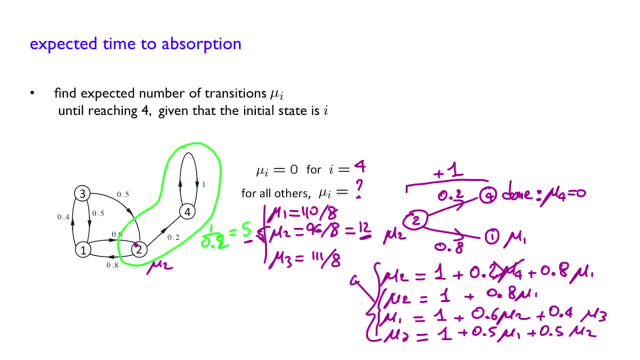 it sort of makes sense: Mu 2,, the state 2, is the one closest to 4.. It is the one actually linked to 4.. So in some sense the expected number of transition to reach 4 will always be the smallest one, because starting. 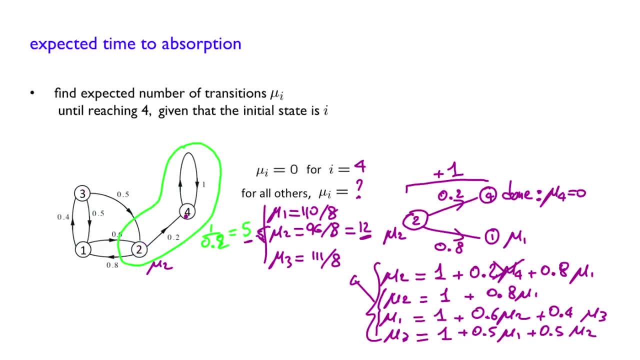 from the other states. you will have to go to 2 before going to 4.. And, in general, if you have a general Markov chain with transient states and one absorbing state and you are asking yourself what is the expected time to absorption, 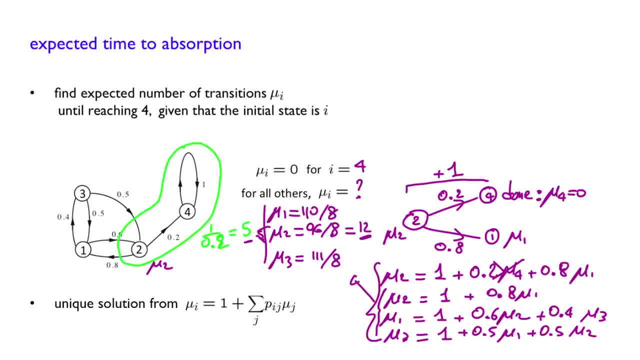 to that unique absorbing state. it will be the unique solution from the system of equation given here, where the pij are the transition probabilities of your Markov chain. Now we have seen how to solve this problem when we have one unique absorbing state. 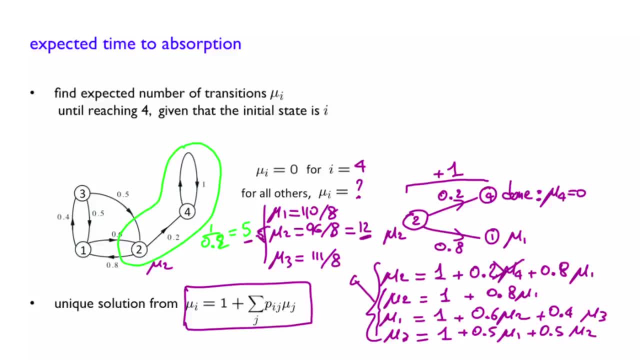 What happens if you have more than one? What happens if you have more than one absorbing state, Like, for example, in this case? Well, first of all a quick note. You realize here that you have 1,, 2, and 3,, three transient. 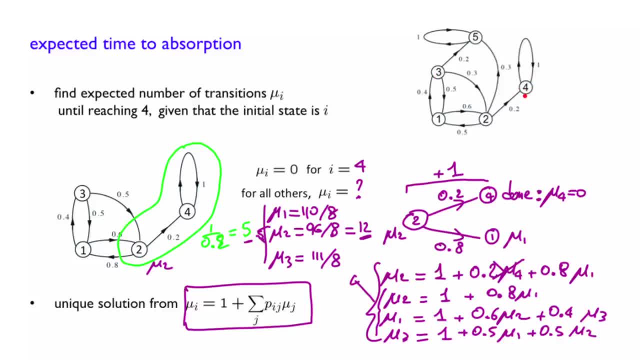 states, And indeed here you have 4 as an absorbing state. It's a recurrent state And once you get to it you stay there forever. And 5 is also a recurrent state, And once you get to 5, you stay there forever. 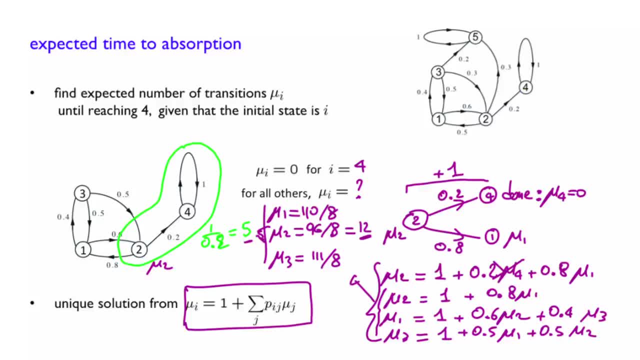 So 4 and 5 are both absorbing states And in a previous video we had seen how to calculate the probability of ending up in 4, as opposed to ending up in 5.. What we know is that the probability of ending up 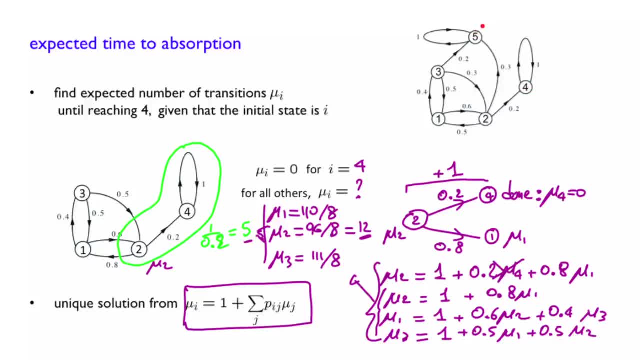 in 4 plus the probability of ending up in 5 will be 1.. But since the probability of ending up in 4 is not 1, trying to find the expected number of steps until you reach 4 specifically does not make much sense. 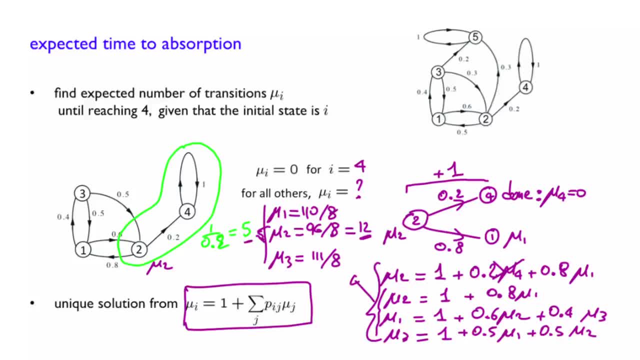 That expectation of that random variable. it's a random variable, but that expectation will not be 1.. It will be infinity. Why? Because there is a positive probability that you will end up in 5.. And if you end up in 5,, once you get there, 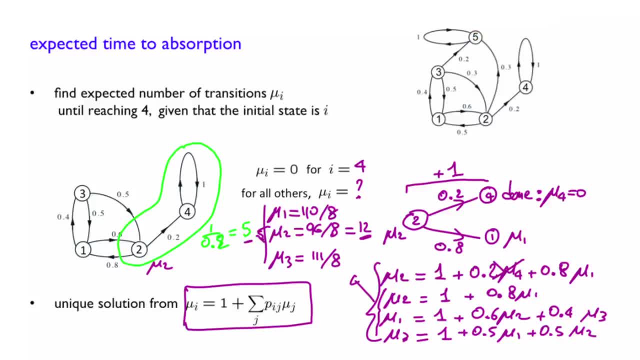 the number of steps to go to 4 will be infinity. So it makes more sense to think about what is the expected time to any absorbing state. so to either 4 or 5.. Now, if you are interested in that quantity, one trick in order to solve that problem, using the technique. 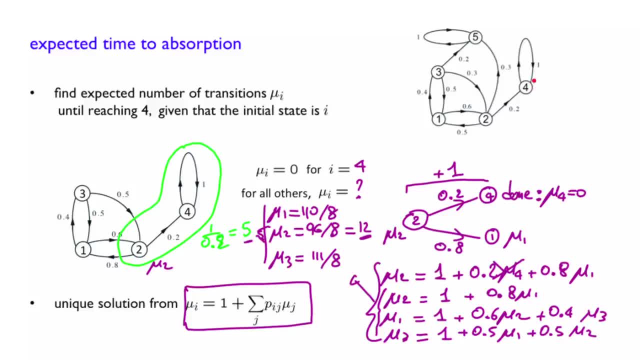 that we have seen so far is to combine 4 and 5 into one megastate, call it whatever- 6.. And 6 is a combination of 4 and 5. It's a big absorbing state And once you are in 6, you stay in 6.. 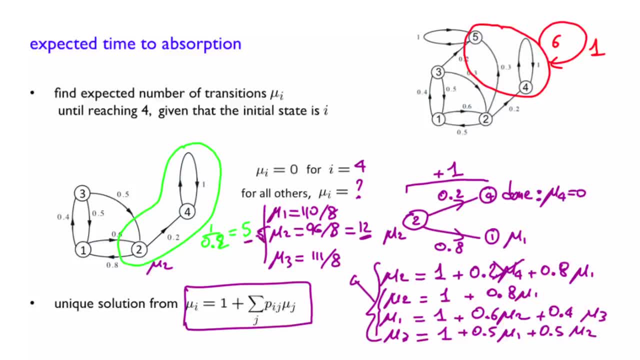 And now you just have to define exactly what is the probability of transition from 1,, 2, and 3 to that megastate. Well, here from 2,. you had originally two arcs. You're going to combine them. You're going to combine these two into one arc. 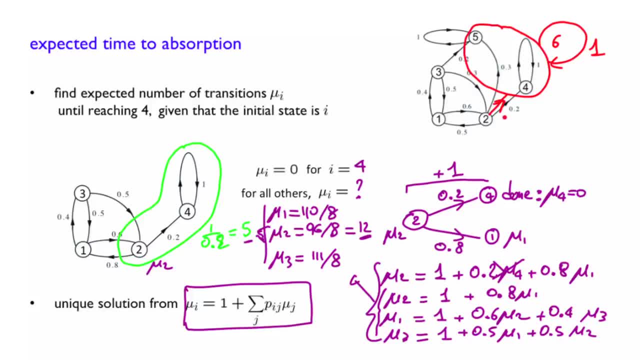 And you're going to sum this probability. So you had 0.3 and 0.2.. You put in here 0.5. And on this arc you had only one arc. So you maintain that arc And you have that probability that you had. 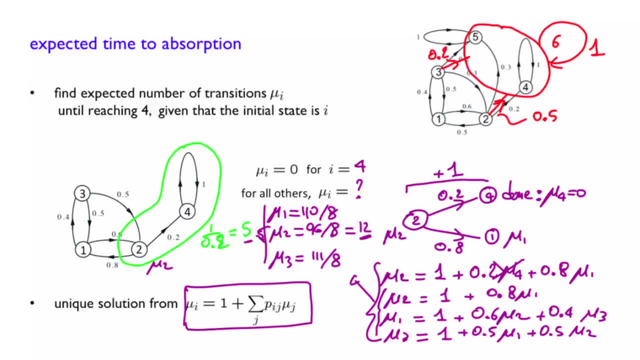 which was, I believe, 0.2.. Now you go back. If you look at the situation now, it's very close to the one here. See this 4 that you have here is this 6.. Now of course, you have another arc here like that. 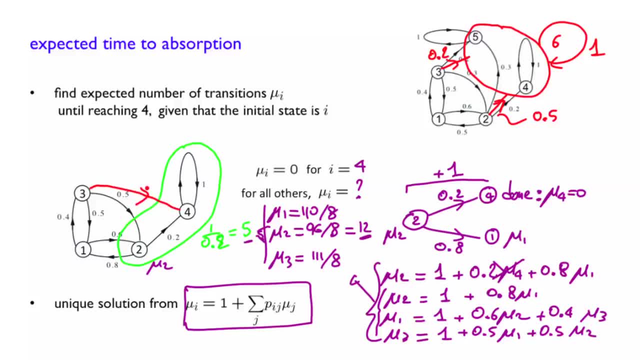 But that's fine, You can still add the arc here and put it at 0.2. And then you reduce this one to 0.3 to make it coherent here. But the idea on how to solve that is identical to this one. 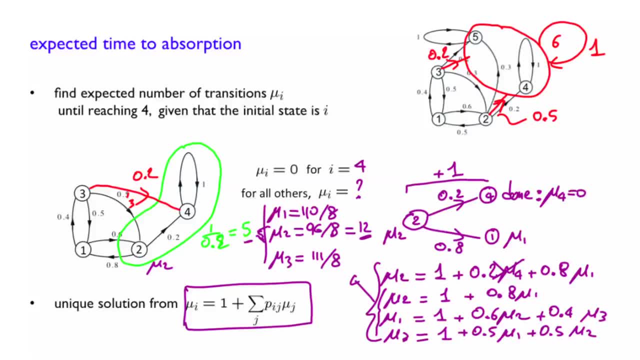 You would have to change a little bit of these, But this is the same technique. So in the end we have seen a technique to find the expected time to absorptions whenever you have absorbing states in an even Markov chain. 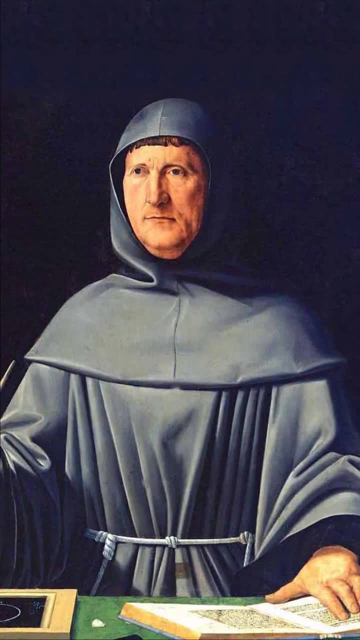 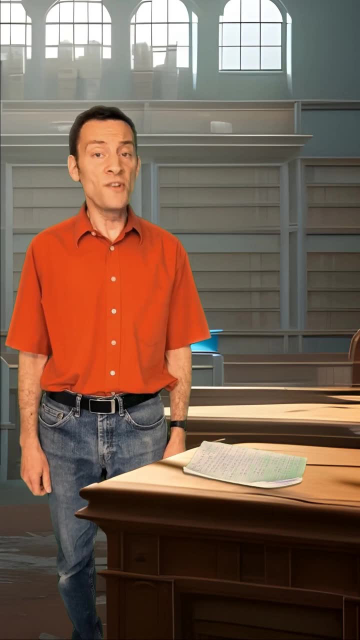 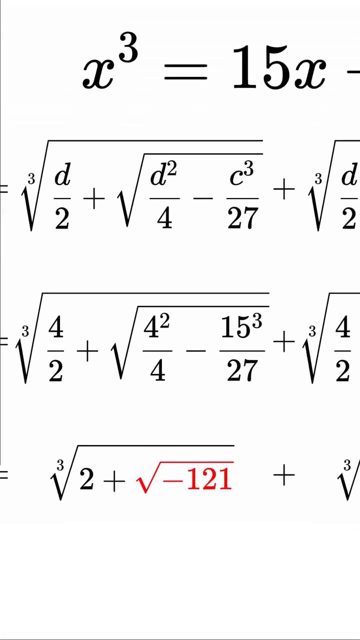 In the 15th century, Luca Pacioli was trying to find a general solution to cubic equations. He finally gave up in 1494.. A solution was eventually found by Girolamo Cardano. However, he came across a few equations that could not be solved as they involved the square.